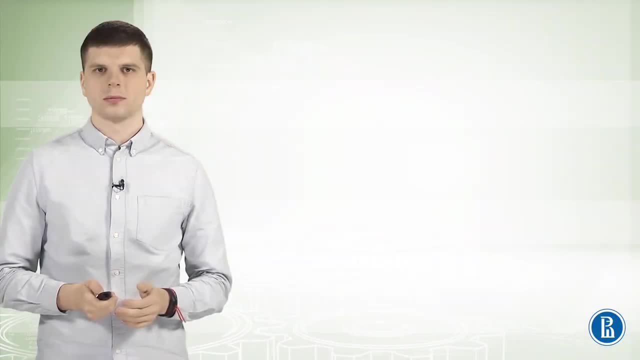 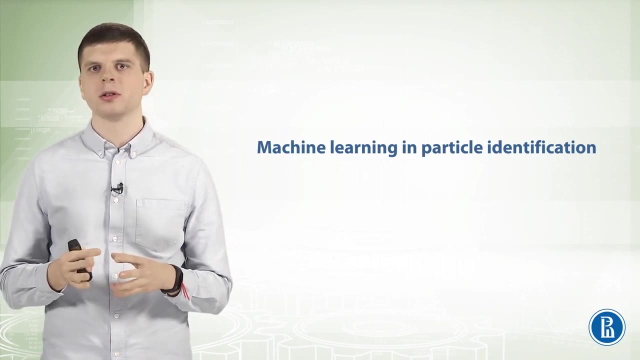 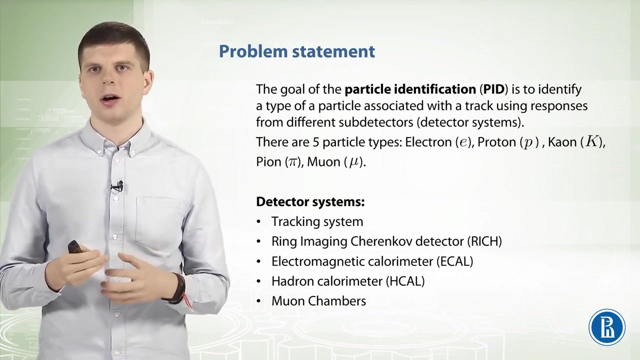 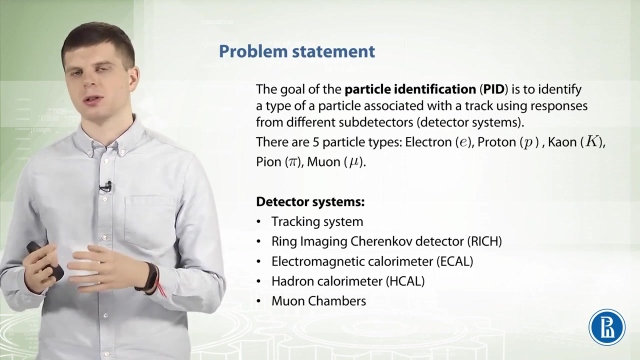 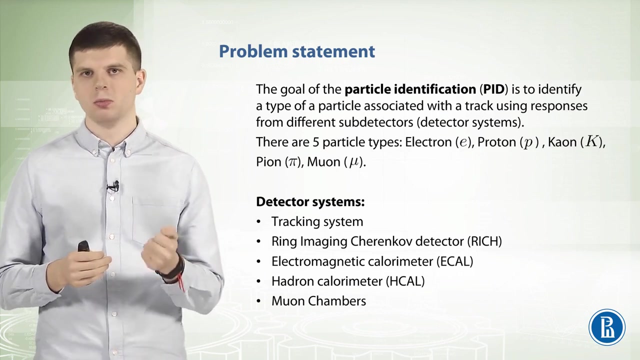 In this video, we will talk about how to use a particle responses in the detector systems for the particle type identification. The goal of the particle identification is to identify a type of a particle associated with a track using responses from different detector systems. There are five particle types: Electron, proton, kaon, pion and muon- And there are five different. 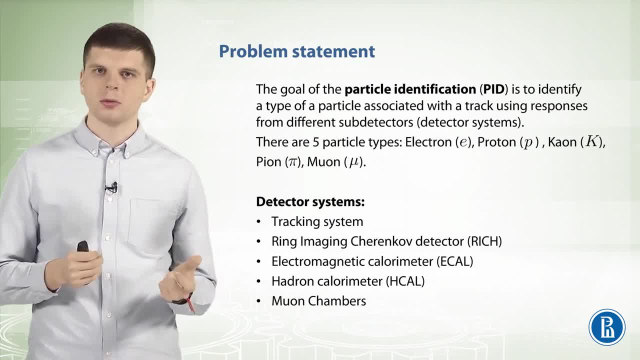 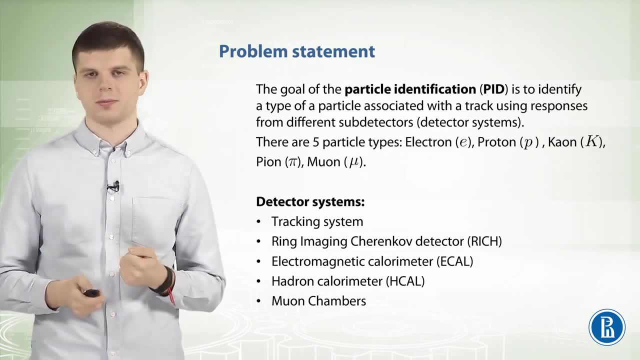 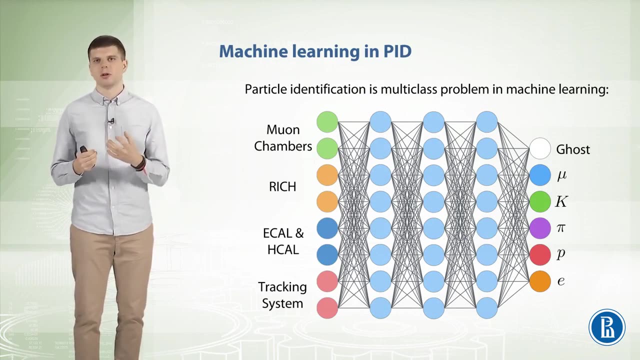 detector systems, Tracking system, ring image, engineering of detector electromagnetic colorimeter and other colorimeter and finally muon chambers. The particle identification problem can be considered as multi classification problem. in machine learning, A particle track responses in the detector systems are used as inputs of a classifier For an example tracking. 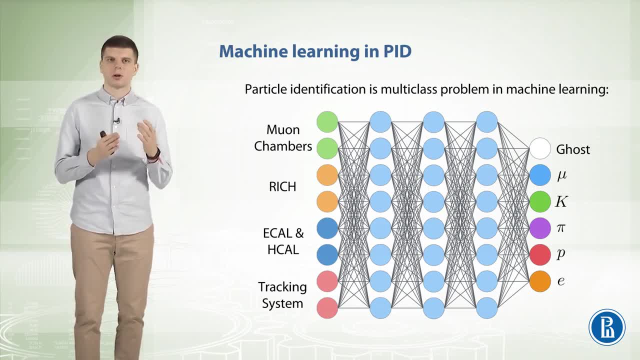 systems provide information about particle track parameters, track fit, quality, particle momentum and charge, and also decay vertex coordinates. Reach detector gives a particle emission angle or delta log likelihood for a different particle type hypothesis. The particle type hypothesis is a quantity of circles fit in the detector. Colorimeters measure particle energy and number. 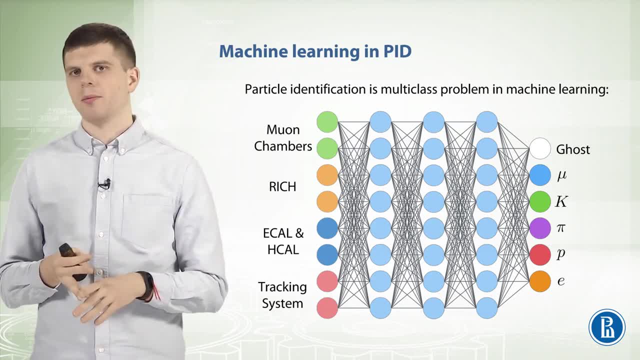 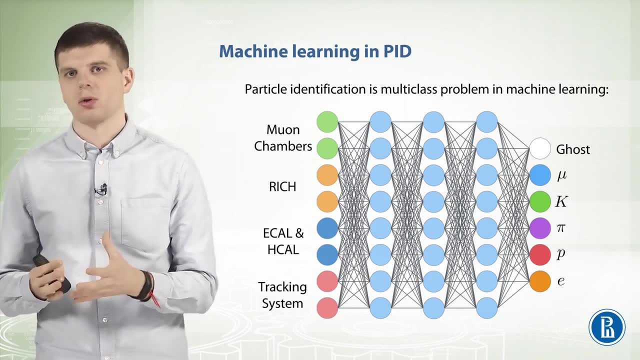 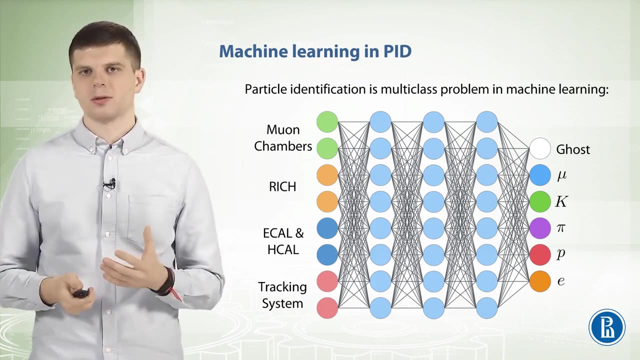 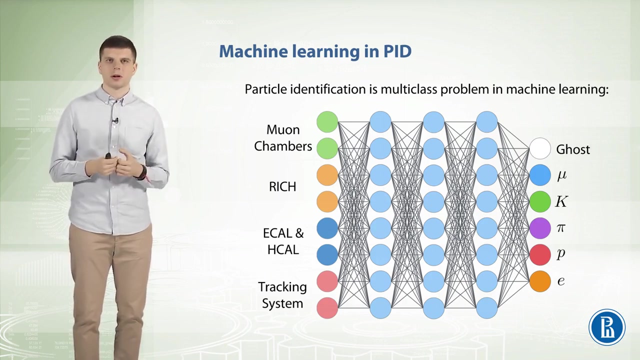 of responses for this particle. For example, muon system tells is a track has hits inside the system or not and how much active chambers corresponds to the track. And there are many other features. Outputs of the classifier are six labels. Five of them correspond to five different particle types: muon, kaon, pion, proton and 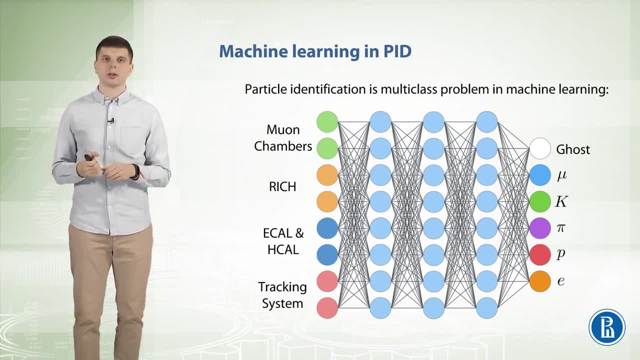 electron, And the last one corresponds to all other particle types and just noisy tracks that are called ghosts. Ghost is a track that was recognized by mistake or the track pattern recognition method and doesn't correspond to any real particle in the detector. So for each track recognized in the detector, the classifier gives probabilities to belong to each of. 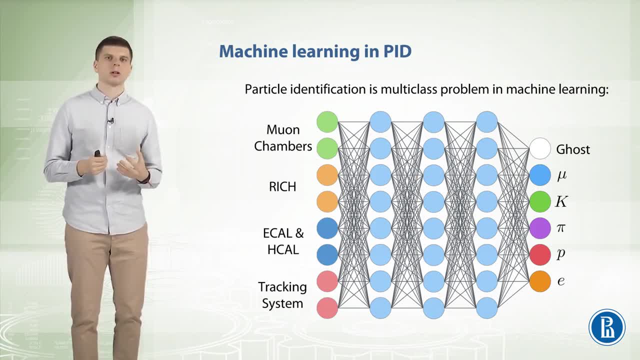 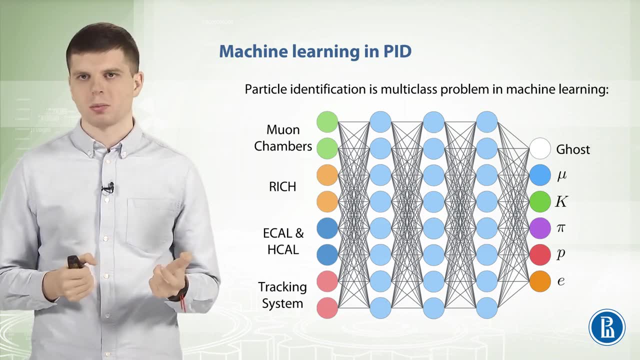 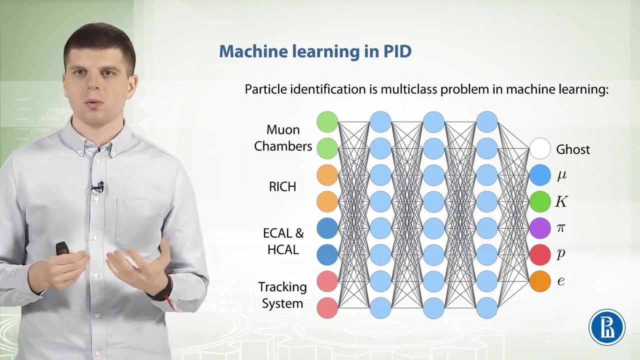 these particle types. This problem can be solved in different modes: in the multi-classification mode, in one particle versus rest particles mode or in one particle versus one particle mode. For example, one particle versus rest mode means that the particle fleet must match its massiece more than one mode. 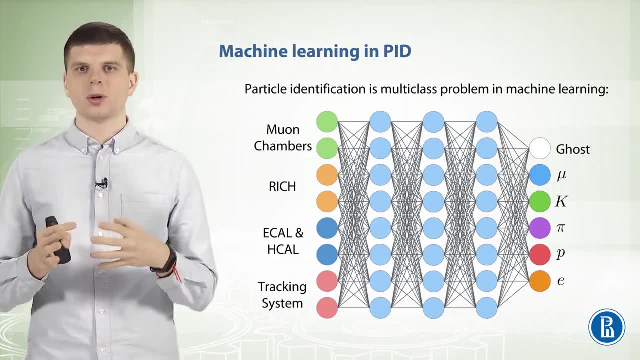 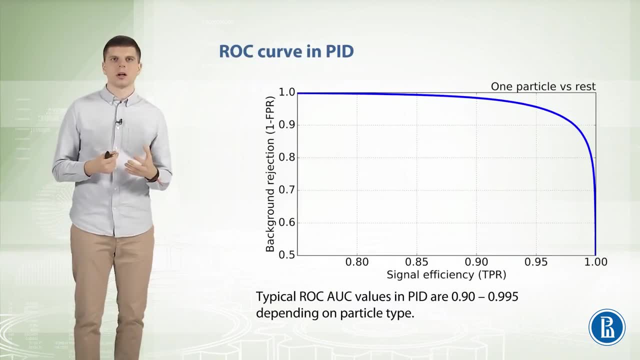 And the protocol size of the particle distribution is simply m, means that you train a classifier to separate one particle from all other particles. Modern detectors in high-energy physics provide high quality of particle identification. In terms of the area under the rock curve, it corresponds to values in range from 0.9 to 0.995,. 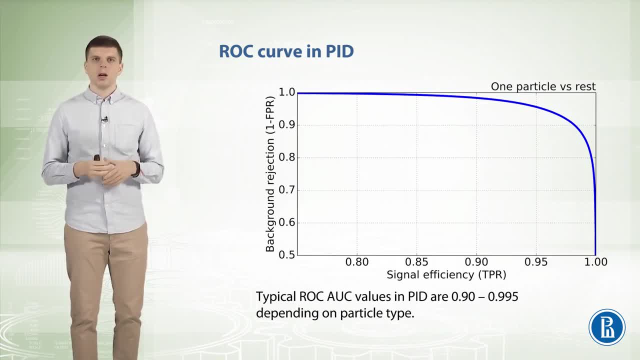 depending on the particle type In your programming assignment for this week, you will be able to train your own classifier for the particle identification using Toi-Montecarlo sample and you will estimate the quality of the identification for each particle type In the machine learning community. 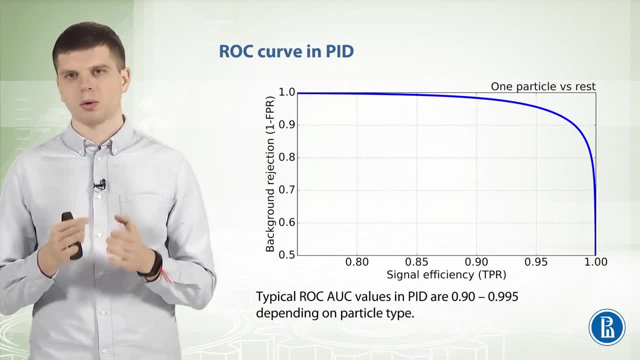 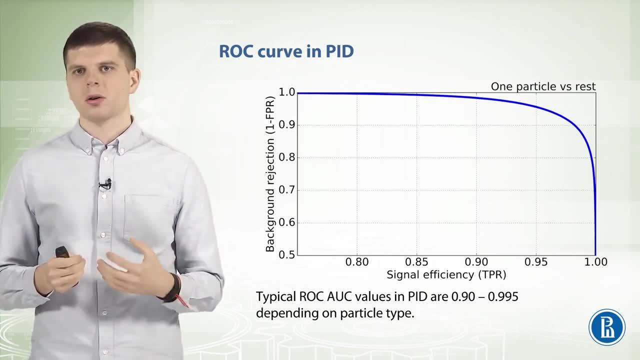 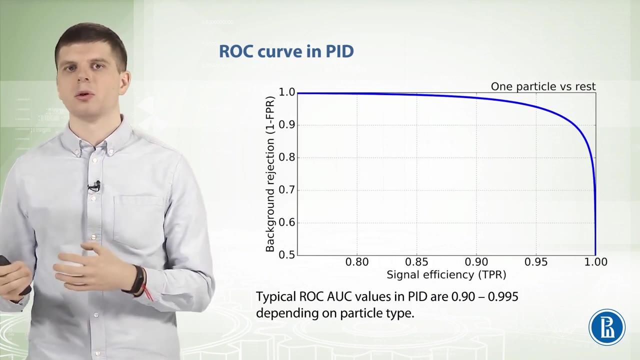 rock curves are plotted as the dependence of the true positive rate from the false positive rate. However, in the high-energy physics, rock curves are easier to identify. Curve is plotted as a dependence of the 1 minus false positive rate from true positive rate. 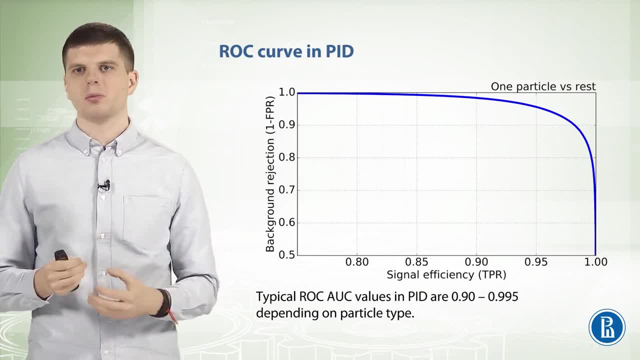 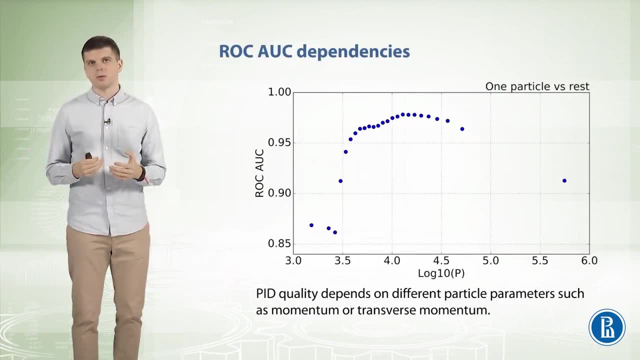 1 minus false positive rate is called background rejection and true positive rate is called signal efficiency. Quality of the particle identification depends on particle parameters such as its momentum, transverse momentum or energy. The figure on the slide demonstrates strong dependency of the area under the rock curve. 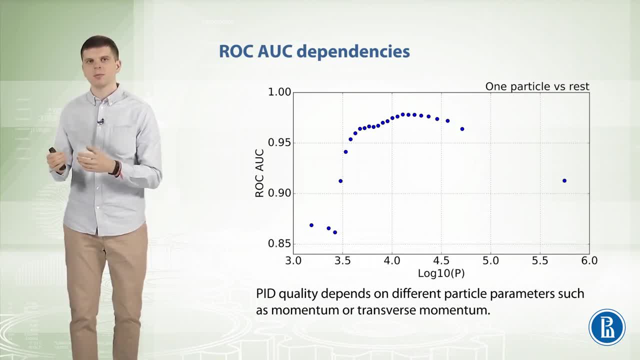 for a particle type separated from all other types from the particle momentum. The quality significantly drops in low and high momentum regions. Moreover, it's preferable to have no such dependencies. In other words, we would like to have flat or uniform dependency of the particle in the